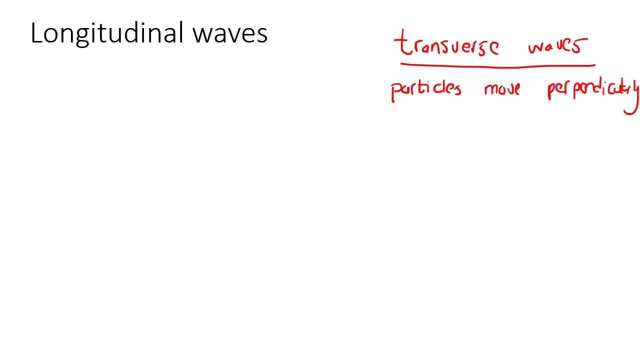 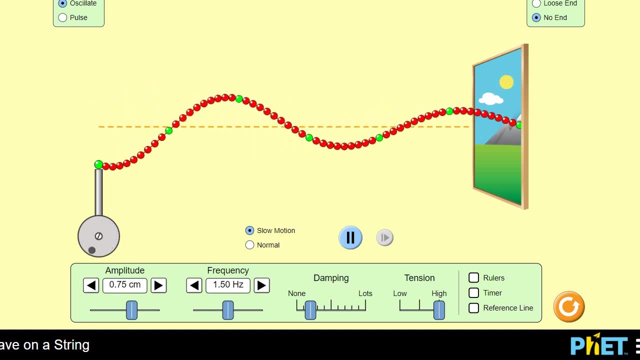 to direction of wave, And so here was the simulation that we've looked at in previous lessons. So, for example, if you have to have a look at this particle over here, I want you to, I'm going to push, I'm going to fast forward a little bit and I just want you to watch that. 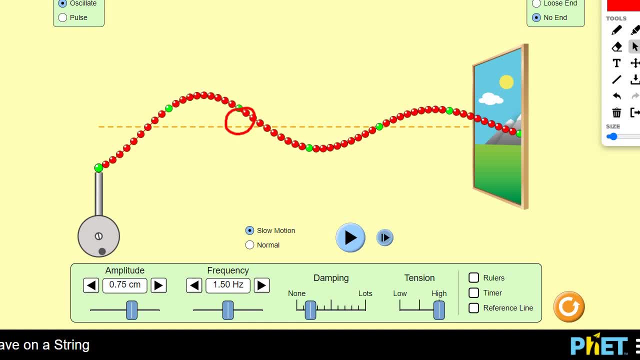 particle, Okay, so have a look what it does. You see how that particle is just going up and then look what it does now And then it goes down. But if I had to show you the wave, you would think that the wave 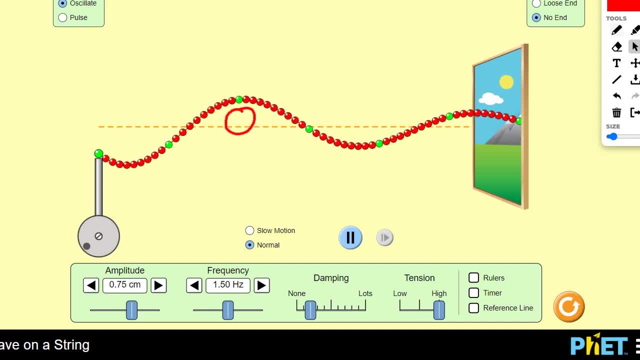 is going to the right. Can you see that? Well, the wave is going to the right. So the wave is going like this: we can see it's moving to the right, Okay, but the particles are just going up and down, And that's what we called transverse. This is transverse, But 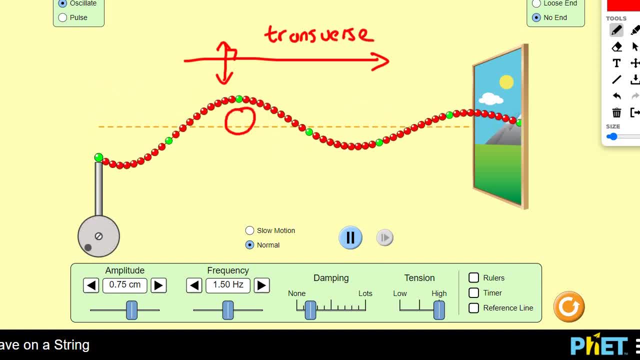 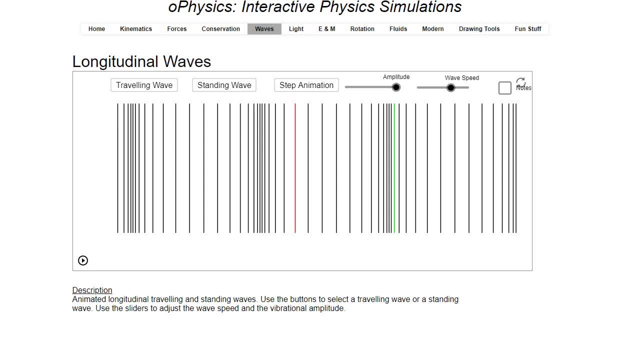 now in this lesson we're going to be looking at longitudinal, which is a totally different type of wave wave. so here we're going to look at a longitudinal wave. now I'm going to let this wave go and I want you to try to see in which direction the wave is going, okay? so if you just look at this, I know it. 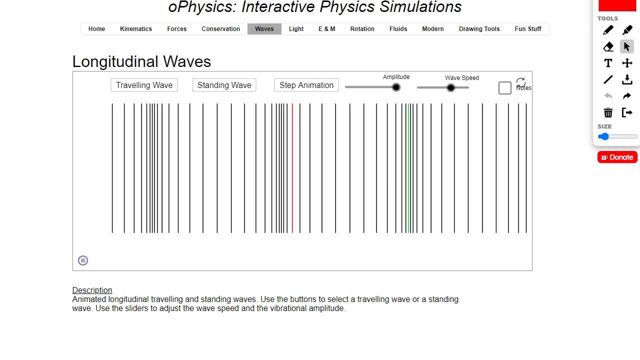 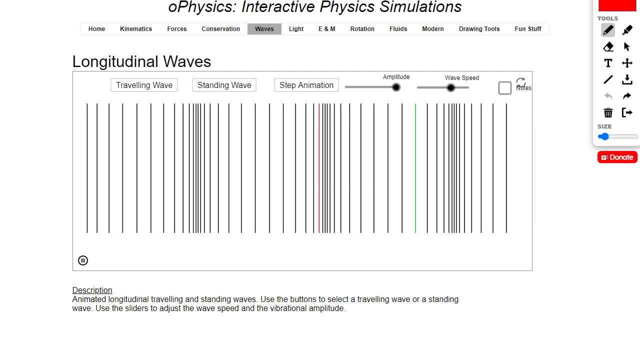 looks really weird, right, but this is a longitudinal wave. now, can you see? we can see things are moving all over the place, but can you see that it looks like the general direction is that this wave is moving to the right-hand side. I mean, just look at this black bar here. now it's over here now. 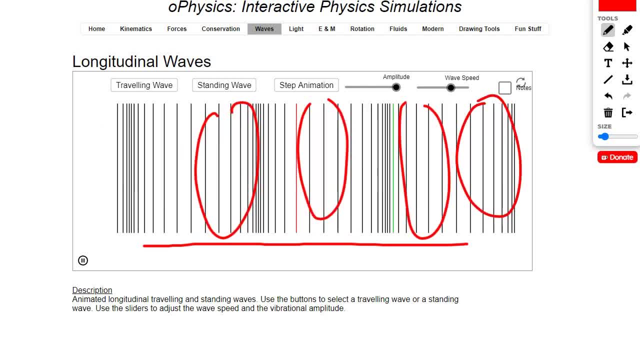 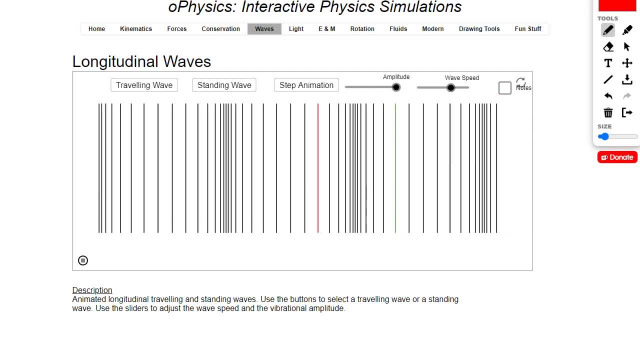 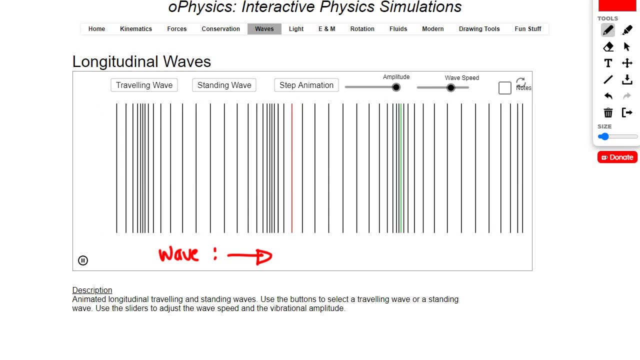 it's over here and now it's over here, so it looks like the wave is going to the right. okay, you can see, everything seems to be going to the right, so we can just say: here, wave is going to the right. now we're going to look at each of the particles, so I want you to specifically focus on this red. 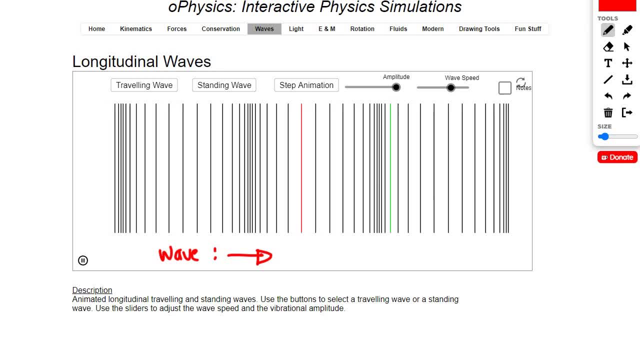 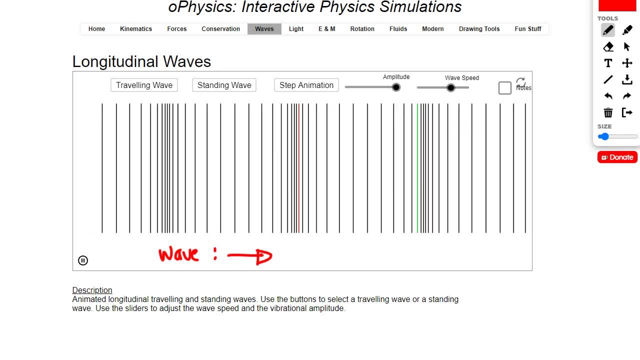 one. look at that red one, okay, and just keep following the red one. what is that red one doing? is it going to the right, or there it's going to the right, now it's going to the left, now it's going to the right, and so it doesn't seem to be moving out of its position. so, for example, it: 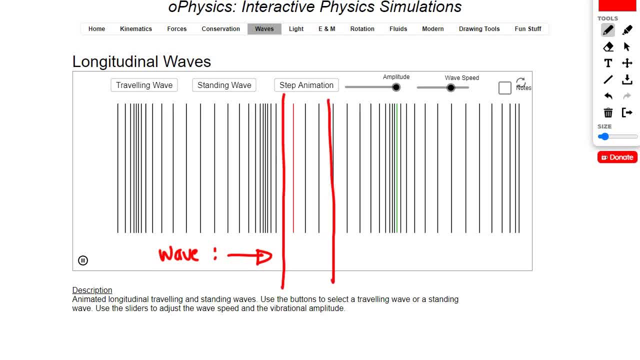 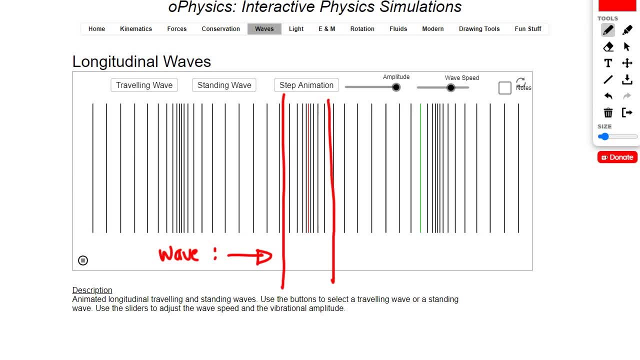 didn't go further than that, and it didn't go further than that. let's see if it ever goes beyond those two points. it never does, and so what we can see, though, is that the particles are moving to the right, and then they're moving to the left. you can also look at this green one if you want to. 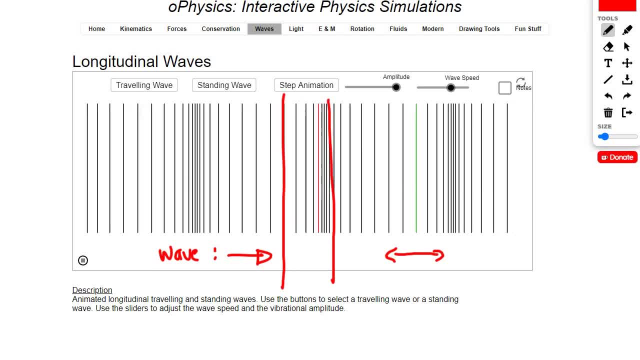 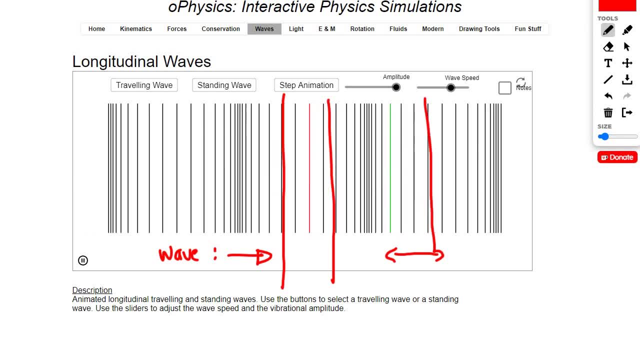 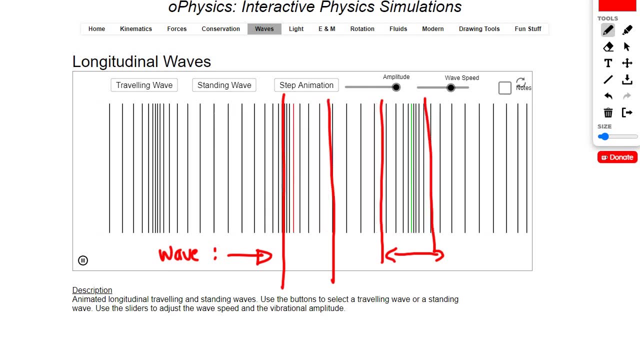 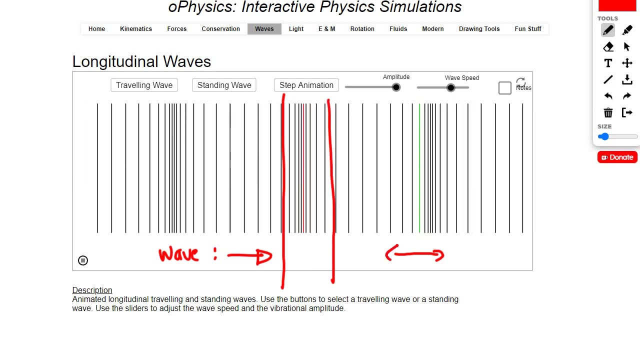 the first position on the right is over there, and the furthest position that it reaches on the left is over there. Now let's see if it ever goes outside of that. No, it never does. So this is what makes longitudinal different to transverse, because what we have now is a wave that's moving. 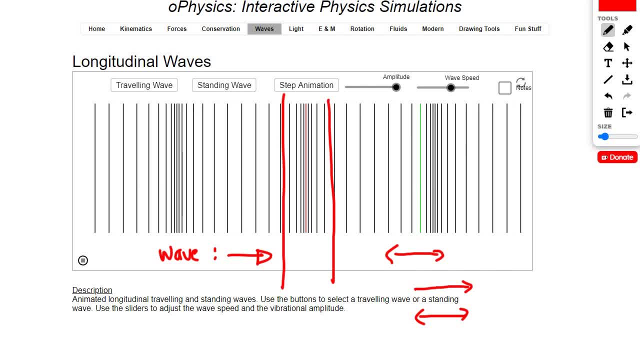 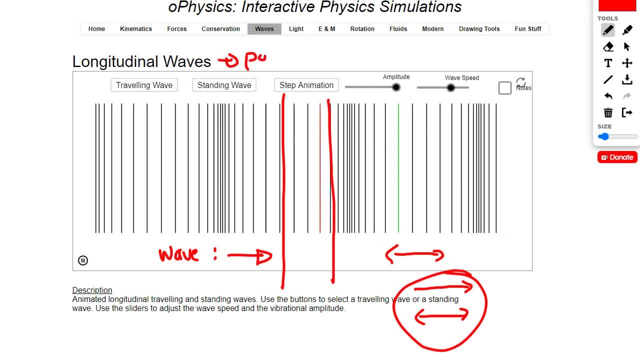 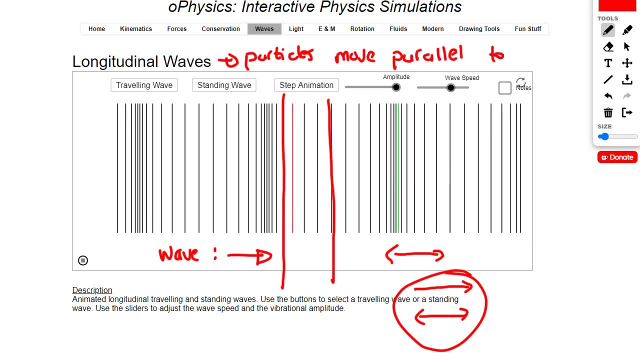 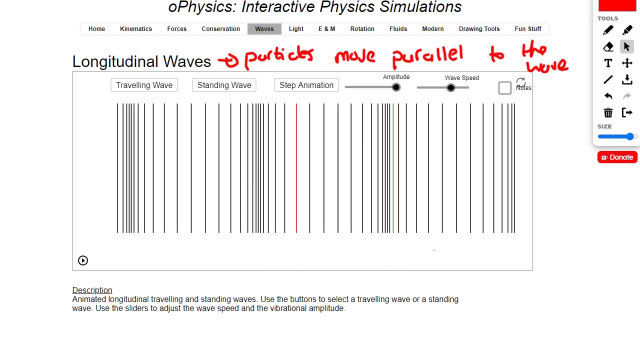 to the right and the particles are moving in the same type of direction. They're not moving at 90 degrees, and so when you have a longitudinal wave is when the particles move parallel to the wave. Okay, now there's some interesting things we need to talk about. All right, so let's talk. 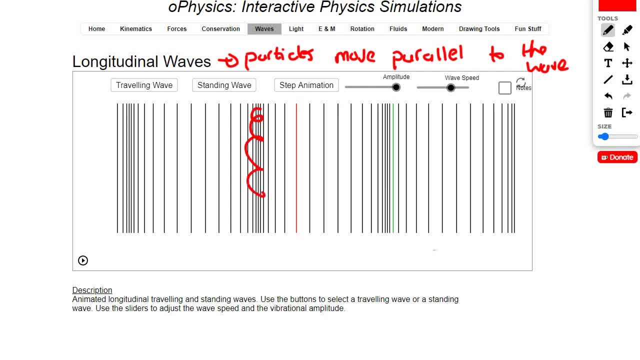 about a few things. This area, here and here and there and there, You see where all the lines are really squashed Or they're very close together. Well, that area is called a compression, because all the particles are compressed together. Then there are areas where the particles are really wide and that 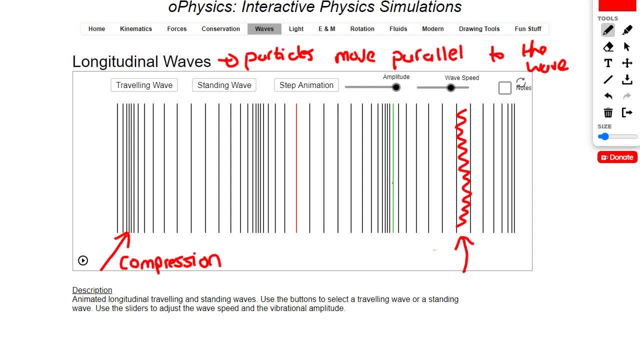 would be like this area over here, Where they are very wide, is called a rare fraction- Very weird word. So the compression is the place where the particles are compressed. So the compression is the place where the particles are close, and then a rare fraction is the place where the particles 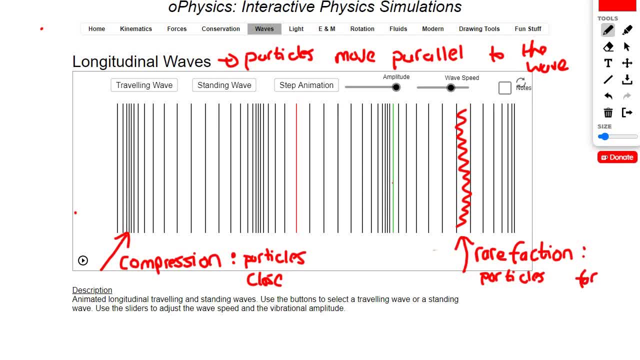 are far apart. Okay, now, if you go connect any compression to another compression, So for example, that to that, That is going to be a wavelength. Okay, that would be one wavelength. You could also go and connect a wave length to a wave length. So if you go and connect a wave length to a wave length,